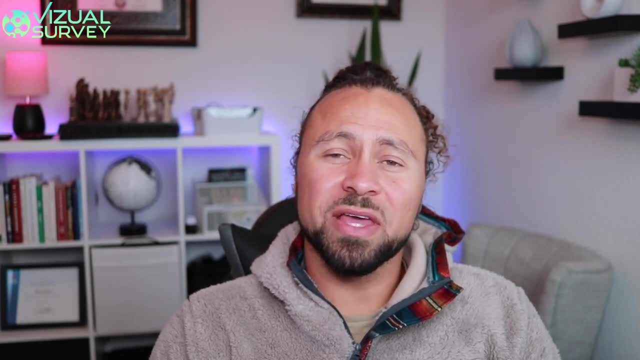 people messed up a little bit because you have that thing where you have to count distinct respondents in order to get the correct count, because one person can answer the question more than once, and that will mess up if you're trying to count rows. Now in this video we're going to show you three different. 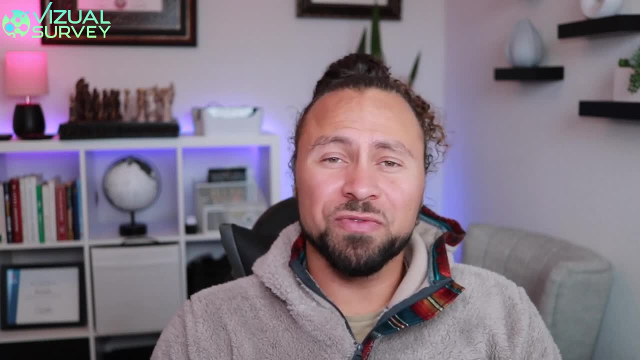 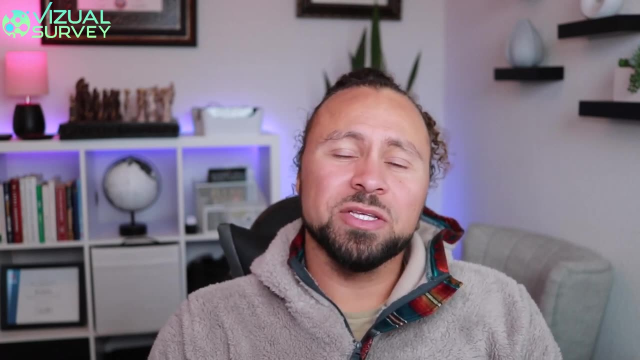 ways to visualize this- multiple-choice questions in three different charts. I'm going to show you how to analyze multiple-choice questions and charts, then also talk about the caveat of how to get the correct percent of total when using Tableau. So if you end up liking this video, please subscribe and like this video, because we will. 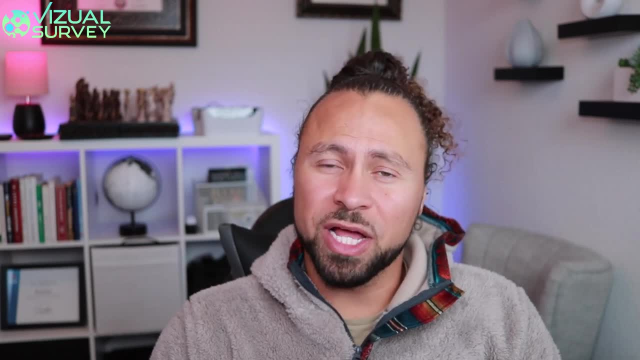 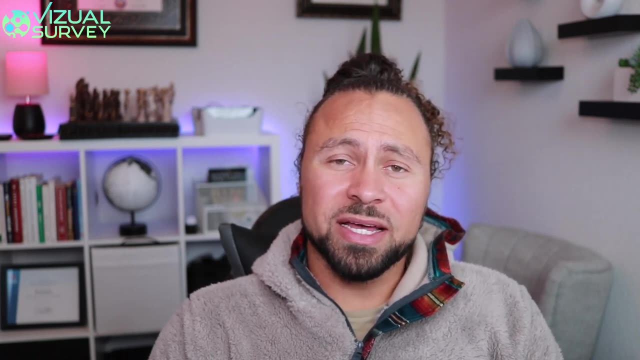 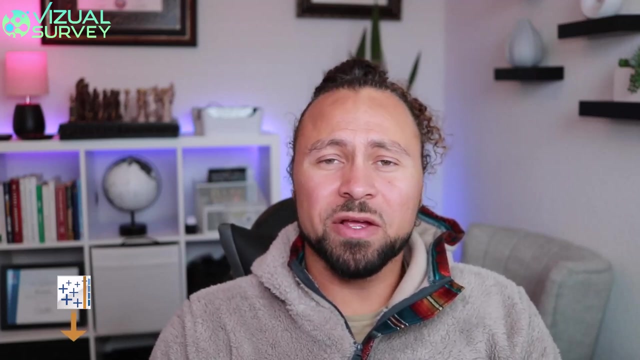 be creating a lot of more videos around how to analyze and visualize survey data and create some cool dashboards. Now, if you would like to follow along, there is a dashboard template that you can download using the link below, so that we can start at the same point and create these charts. 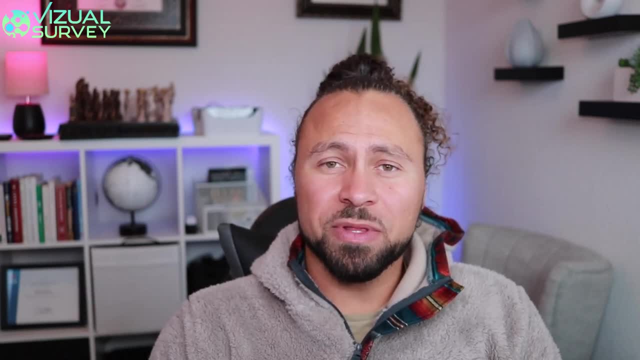 together. Now, the data that is in the dashboard template that you will be downloading has already been ran through Visual Survey, so you'll notice it's in a very nice, clean format, already structured perfectly, and it's not in that kind of wild wild west format that you get. 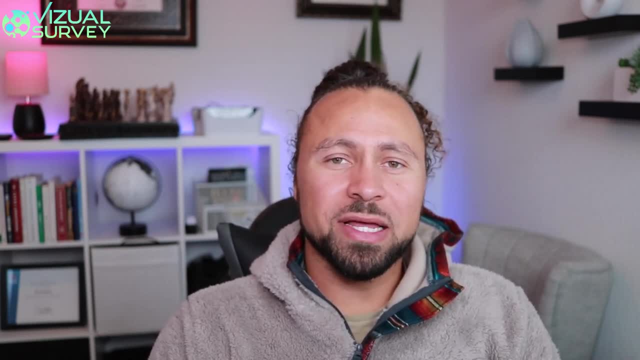 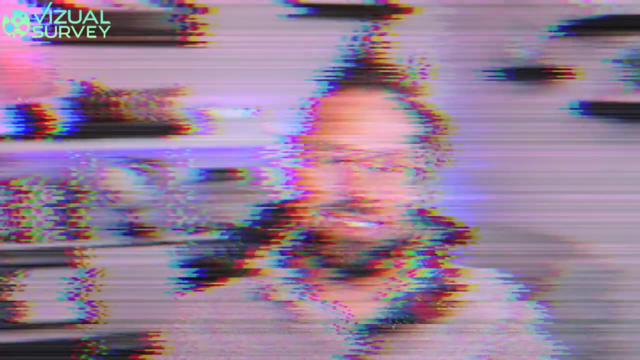 out of survey platforms, So we will be working with already cleaned and transformed data. As you see, it will make things a lot easier. All right, let's go ahead and jump into the video. I'll see you there, All right, so let's go ahead and jump into the video. 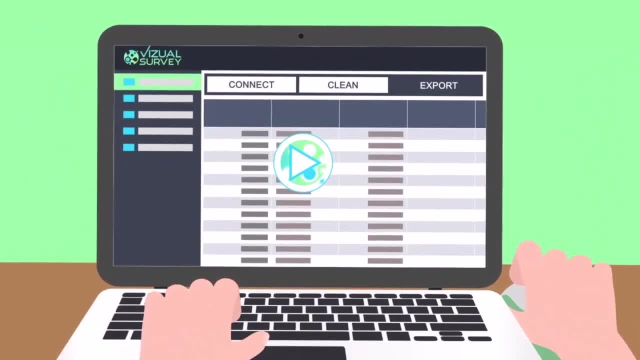 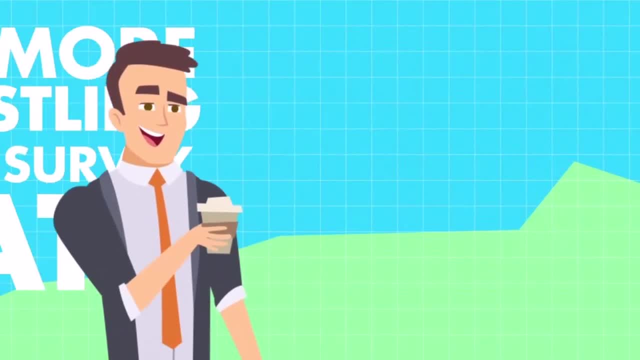 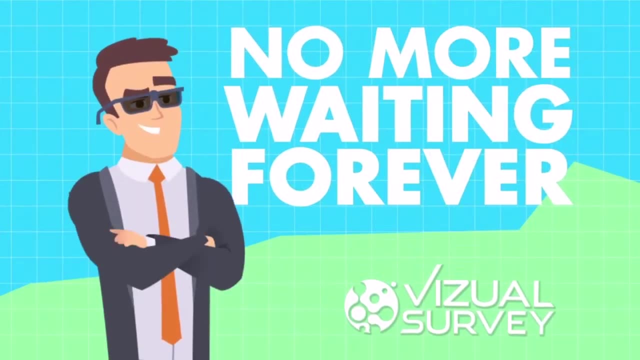 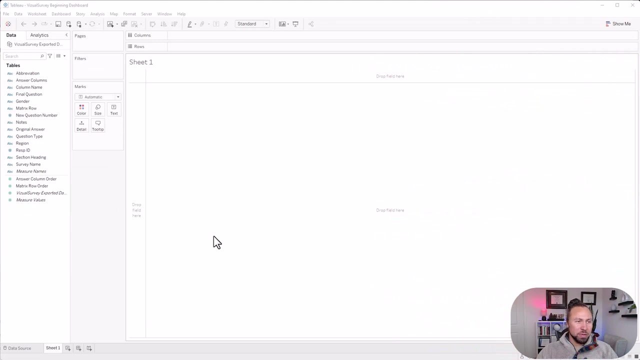 All right, here we are in the Tableau beginner file. Like I said, if you don't have this file, download it. It will have the data already preloaded in it so that you can follow along In this video and create these charts with me. 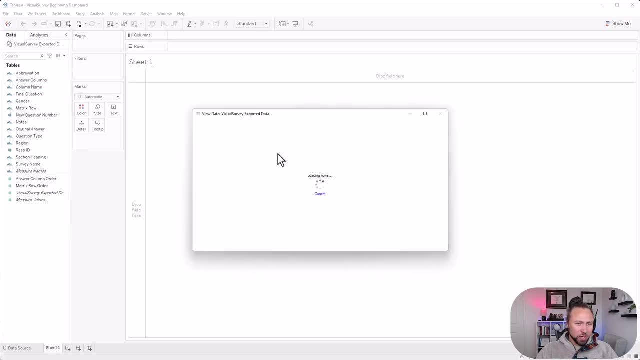 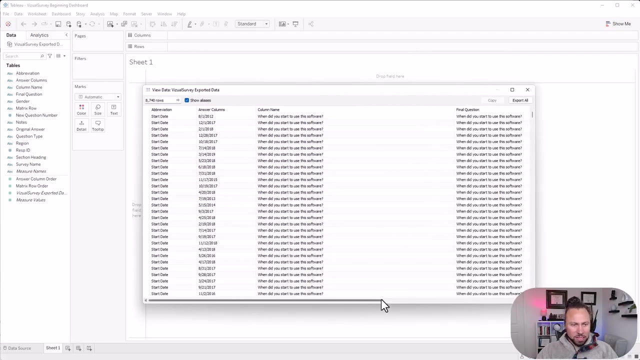 So first thing we want to do, So this data I'll show you real quick. Like I said, it's already pre cleaned because it's been run through Visual Survey. So we created this cleaning methodology that gets this data exported in a perfect output. 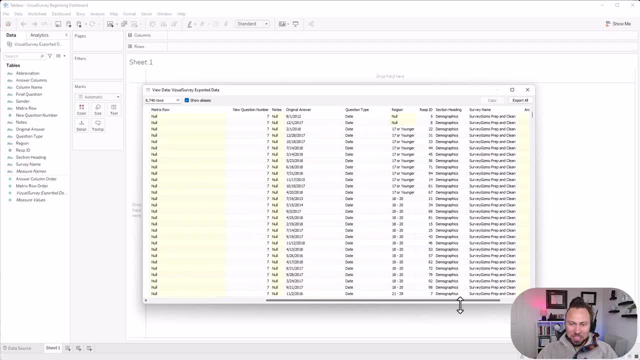 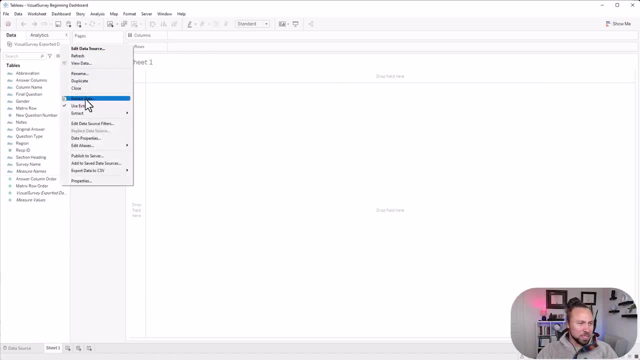 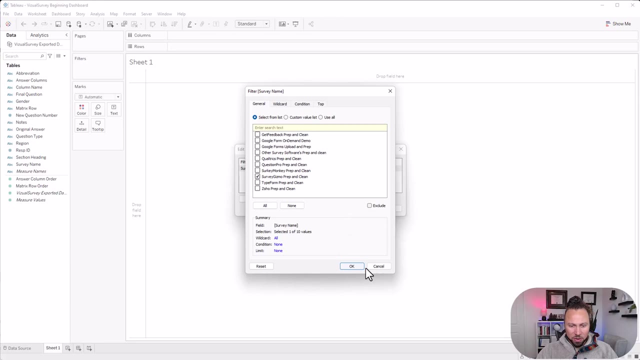 So actually you'll notice there is multiple surveys in here from multiple survey platforms, So we got some survey, gizmo data we have. Let me see If I go to data filters. so Google Forms, so Question Pro Type Forms, Zoho: Get Feedback. 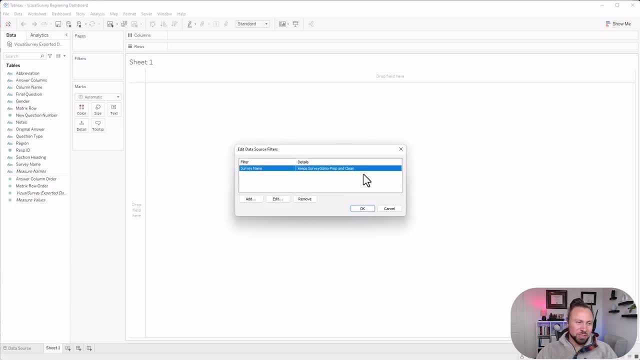 all that. So there's actually a whole bunch of surveys in here from different survey platforms that we ran through the software, But on this one we're just going to look at the survey gizmo data. And then I have all these standardized columns here that we use to help us create the visualizations. 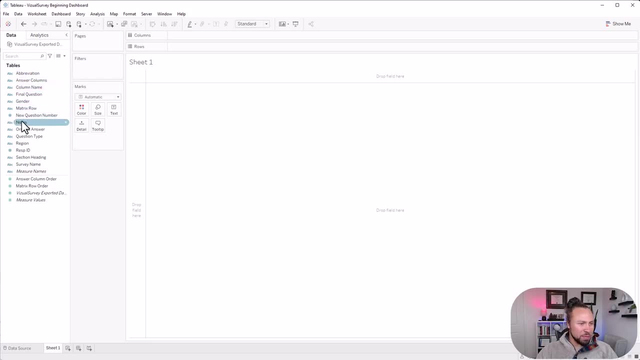 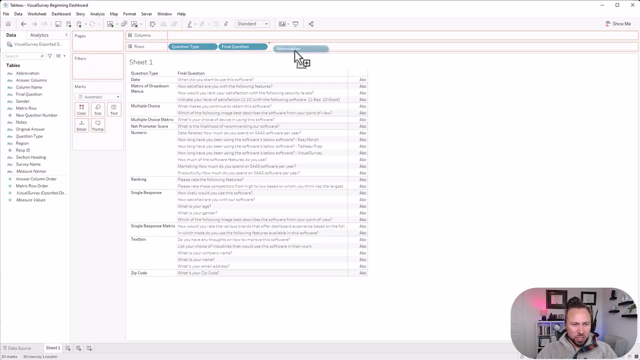 All right, so in here we're going to first grab our question type So we see what kind of question types we have in here. Let's grab our final question, So see all the questions, And then I created a column- or there's a column in there- called abbreviations, like 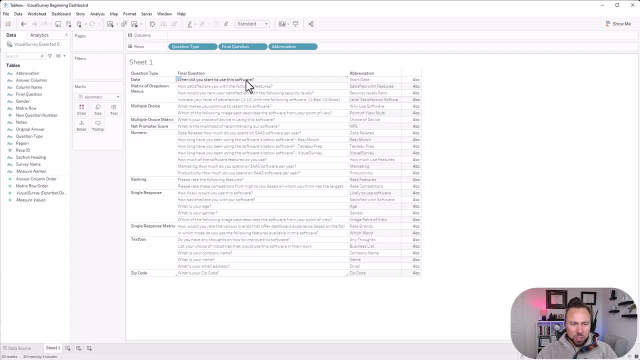 a little short snippet of the question. So, when you start this software, start date, all right. How satisfied are you with the following features? Satisfied with features? Okay, Since we're going to be doing multiple choice, let's just filter to be multiple choice. 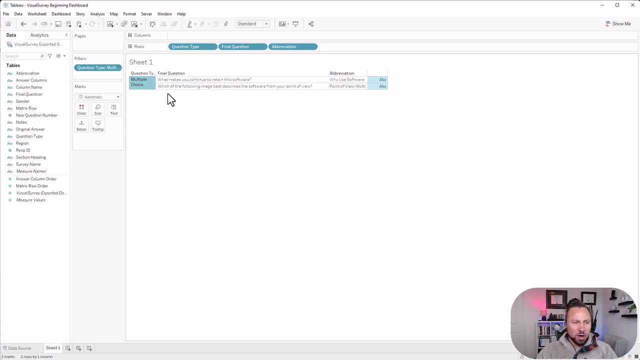 We have these two questions: What makes you continue to retain this software? Which of the following images do you use? What makes you continue to retain this software? Which of the following images best describe the software? I'm just going to use the abbreviation, just so we can keep those out. 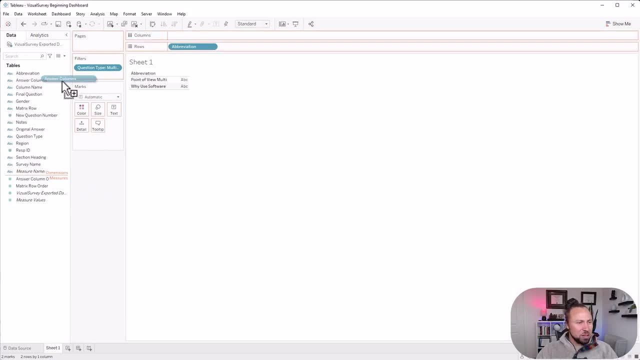 So I'm going to remove these. Now we have our answer columns. Bring that in. We can see the answers for each of these questions. I'm going to get rid of this null, So I'm just going to right-click: do exclude. 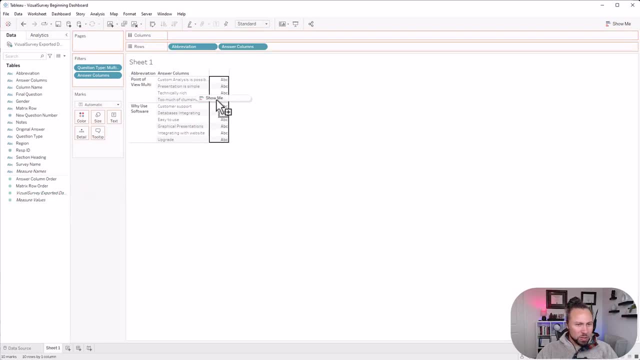 And then now we can bring in our rows. okay, So now these are the number of respondents that answered these questions. Now for questions like this, where it's multiple choice, if we try to do a quick table calculation- percent of total- then it's not going to give us our right percent of total because this: 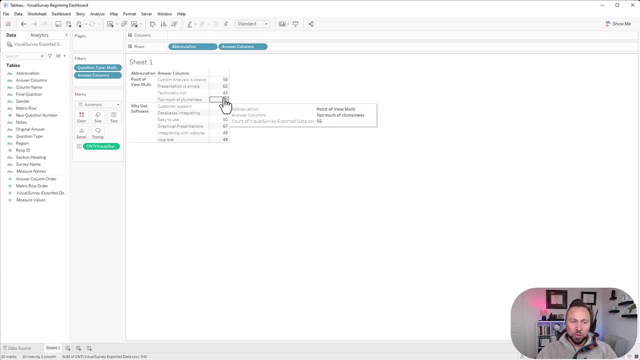 is all going to add up to 100% compared to if we do it with distinct respondents, And that would make more sense once I show you okay. So first thing I'm going to do is do the calculated field and create it. So I'm going to create calculated field. 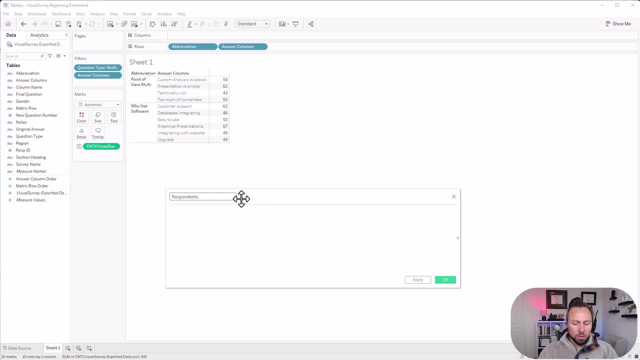 And this is respondents. Okay, All right. All right, So I'm going to do this, And it's a count D, it's count distinct of our responded ID And I'm going to bring that in. All right, Now it's going to be the same number for now, right. 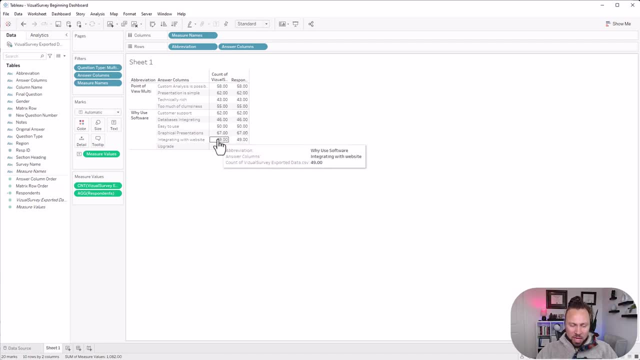 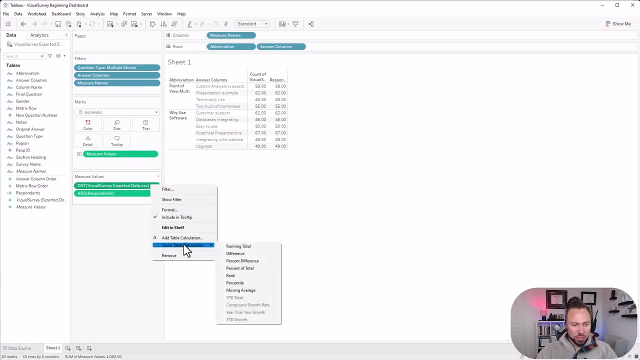 Because we're counting essentially rows right here. Where the difference lies is when you try to do a percent of total. So this measure here is just row count. If I do a percent of total with this right, it's going to give me a percent of total currently. 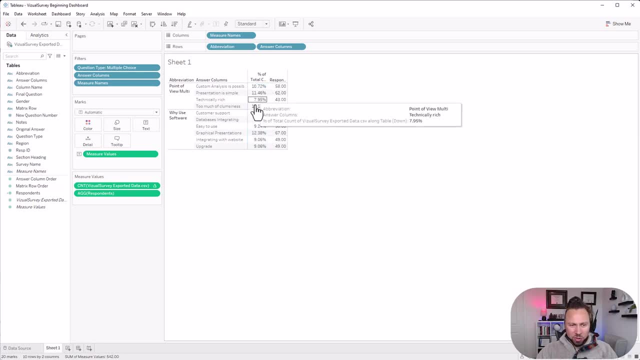 it looks like it's doing. all of these are percent of total, but I want it to do a paying down And then it's going to give me: this is a hundred, So it's going to reset per question. Now, if I do respondents and I do a percent of total, make sure it's paying down. 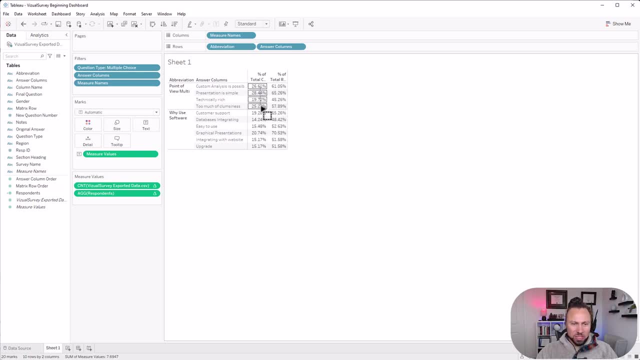 You see the numbers are different because this is row count. So this is going to add it to a hundred percent. but for multiple choice questions it's not going to always add up to a hundred percent. it's going to usually be more because one 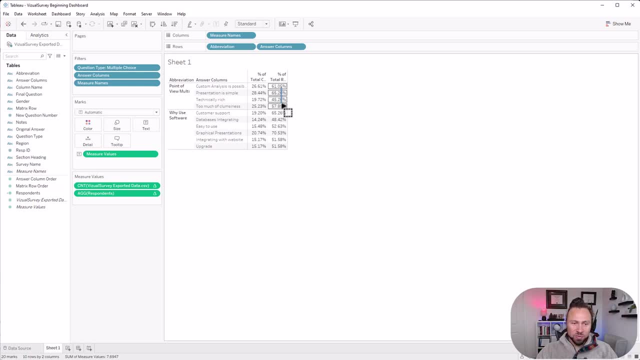 person can answer that question more than once. So this is the real count, because because you can have, like I said, one person answer the question twice or three times with different answers, So you have to do this responded ID one to get the true value. 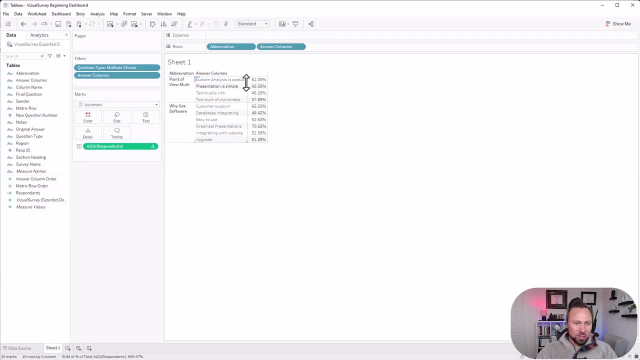 So I'm going to go ahead and get rid of this, Okay. So here's the questions, Here is the answer columns, Here's the percent of totals. All right, And another thing I like doing is bringing out my abbreviation as a quick filter. 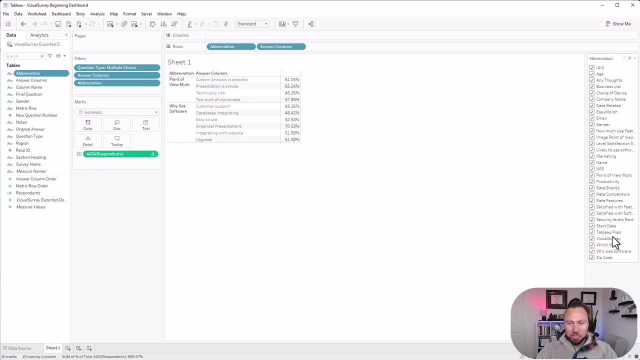 So I'm a right click show filters. All my variations for all my surveys are for all the questions are right. here I want to do the only relevant values And I'm also going to make this a radio, all right, so that I could pick between my two. 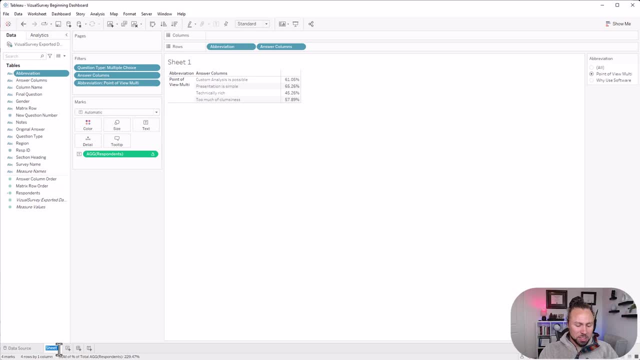 questions. All right, And I'm going to call this my data table, All right. so now we got the basis done. Now this is the important part. Now, from here, we do the chart building. So I'm just going to right click this tab. 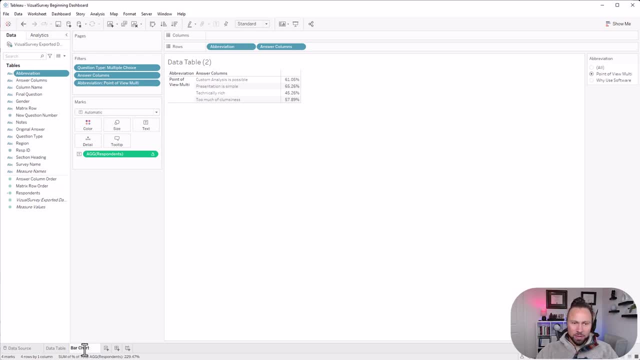 And I'm going to do a bar chart for this one. All right, everybody loves bar charts. bar charts are the most popular thing in Tableau, because they're really the most powerful. So what I'm gonna do is I'm going to get rid of abbreviation. 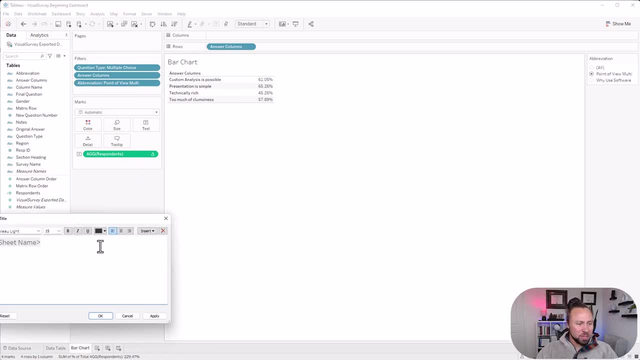 Okay, Okay, Here we go. So I'm going to go ahead and I'm going to go ahead, and I'm going to go ahead and I'm going to double click here and my title of a double click here, and you can insert your abbreviation here. 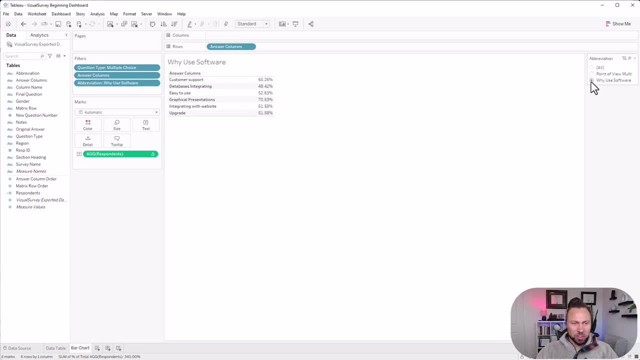 So it shows up at the top. So when you're changing your abbreviation, your questions, you can see that abbreviation at the top. You also put your final question text there. if you want, You just grab your final question text, put it in like the tooltip. 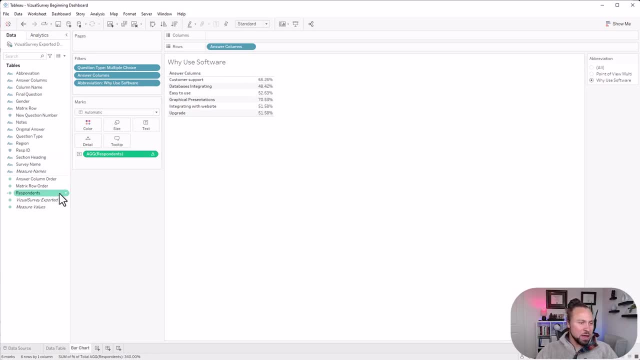 So it's somewhere on the view and then you'll have the option to do it there. Let's just go ahead and do it for fun, just to kind of show you. So go there, bring it in, Bring it in, and instead we can do the final question. 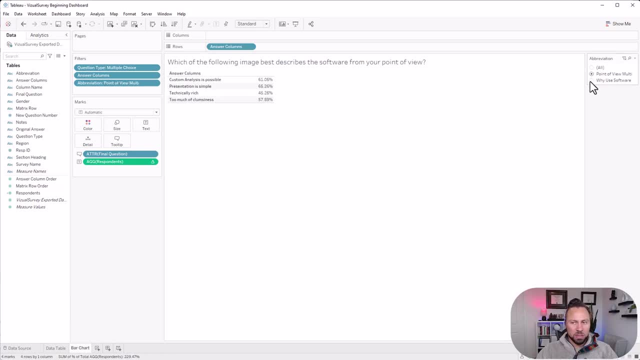 Put one or the other in there, It doesn't really matter, And then the question will go across All right. So now I want to convert this to a bar chart. All right, I want to see my percent of total. So hold control. bring this into the labels. 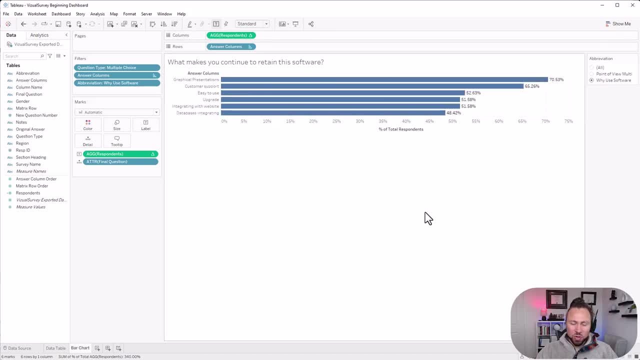 All right, I got my percent of total. Another cool thing to do- especially because you're going to be using this percent of total all the time- is you can make this into a saved calculation. So I'm going to hold control, I'm going to bring this over to my data table and then it's going to ask me to name it. 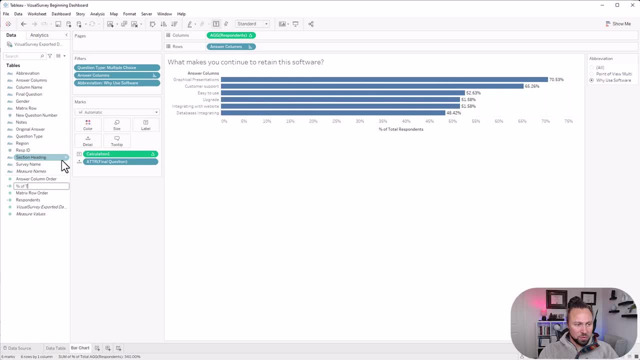 I'm just going to name it percent of total, And now I don't have to do that step every time. I can just use this calculation for everything. Also, you can do a default property and save the formatting as something different. So I'm going to right click default properties- number formatting- and I'm going to do this. 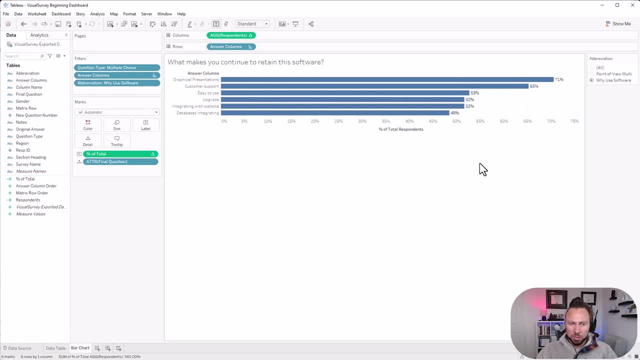 And I'm going to do decimal with no decimal place or percentage with no decimal place. Okay, From here, just kind of clean it up. I like my bars a little thicker. We're going to maybe pick a color for it. I don't like the grid line, so you can right click format. 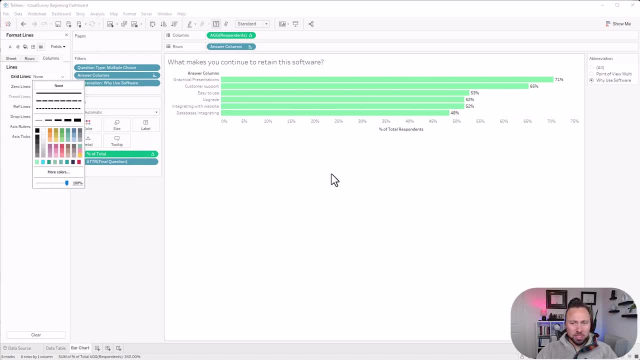 We go to lines, we go to columns, we get rid of the grid lines. All right, We can get rid of this answer column thing here. And you see we've got this question and this question, All right, All right. 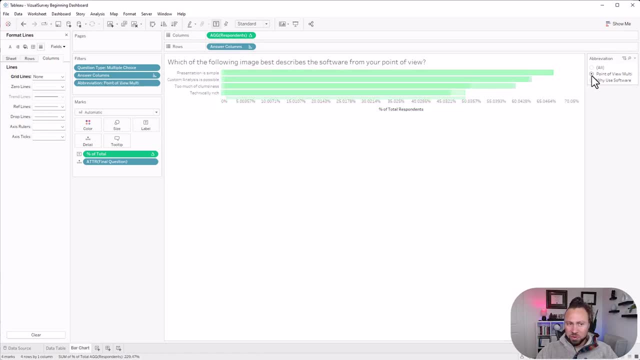 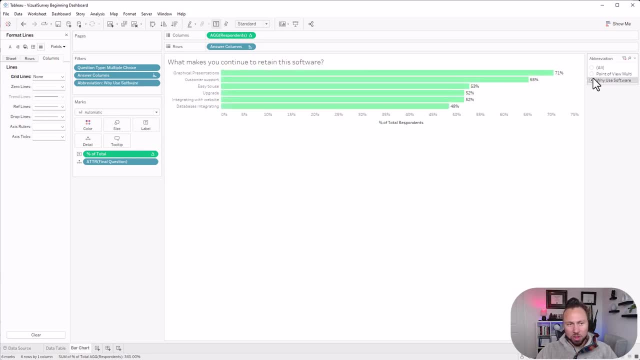 Calculation is all the same. You'll just use the same bar chart over and over again for all of them. You had 50 multiple choice questions. They'll all be listed here and you can go through all 50 of them, All right. 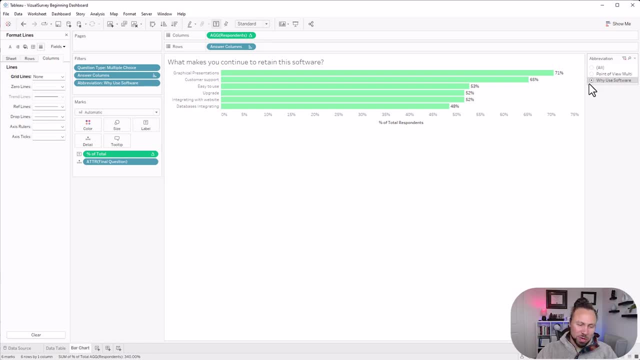 So this is one way you can visualize multiple choice, which is probably the most common. Another way: let's go ahead, and I'm going to duplicate this to kind of just save me a little time. Another way is: This is a donut chart or a pie chart, either one. 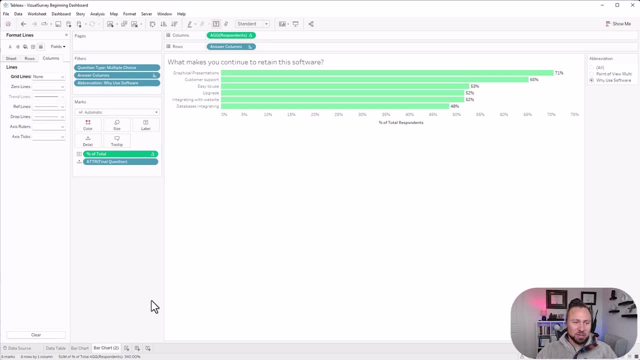 I like donuts so I do a donut chart. you know kind of I guess pie charts are kind of going out of style, But if you put a blank circle on top of it it looks cool. So we're going to go with a donut chart. 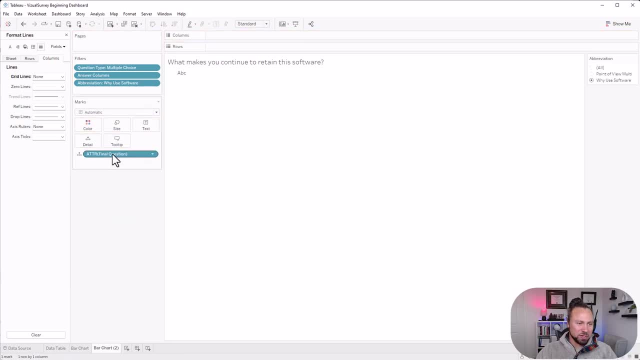 I'm going to just kind of take everything off so that I can kind of create this from scratch. A donut chart is kind of like an intermediate chart type. It's not in the show me, but it's really easy to make. I'm going to show you how to make it. 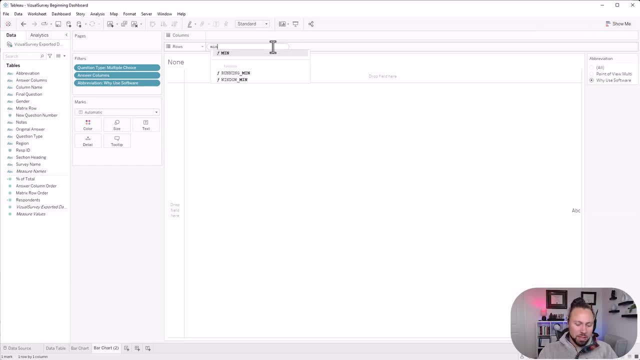 It's pretty simple. but you just double click in here and you're going to type in Min one like that, and essentially I'm doing this just to create two axis, because I'm going to make a pie chart at the top, make just a circle at the bottom, and then I'm going to do a dual axis to put on top to make it look like a donut chart. 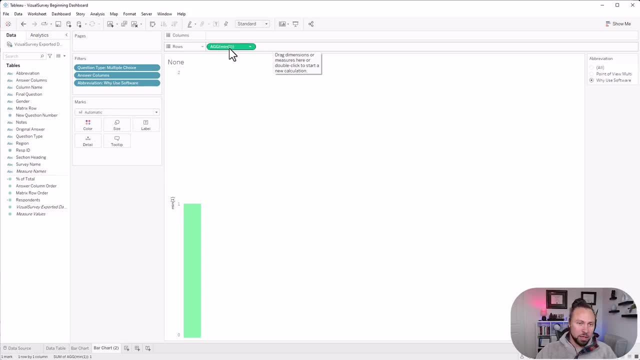 It's not really a donut chart in tableau, but it looks just like it. I'm going to hold control and click and drag this over so that there's two axis, And then now I have these two. I have all, which I'm not going to mess with, but then I have the first one, which is this one: 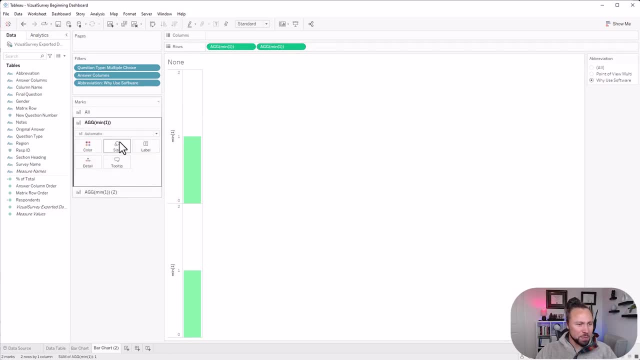 The second one, Which is this one. Okay, so I'm going to go with the first mark card here and I'm going to bring in my answer values. I answer columns into my color. I'm going to change this from automatic to a pie. 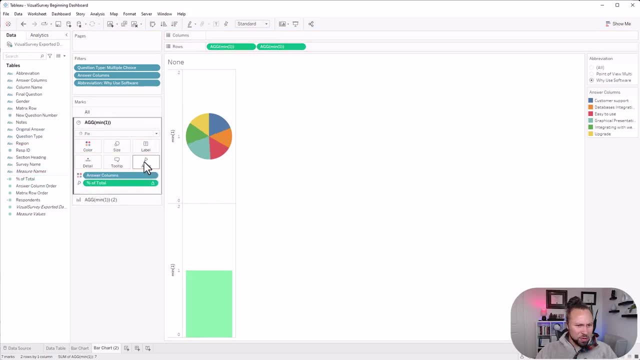 And I'm going to put my percent of total in my angle. That's going to start generating my pie chart. I'm going to do fit entire view so I can see it better. So at the top I got my pie chart going. 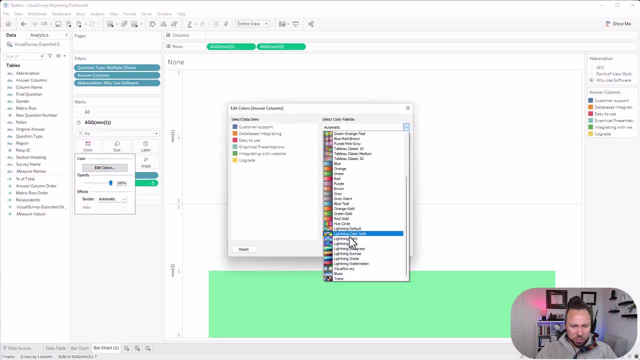 All right, I'm going to change my colors, So I don't like those colors. I'm going to go with visual surveys color palette- All right, so I got the colors there. You can then do some transparency if you like and add some borders. 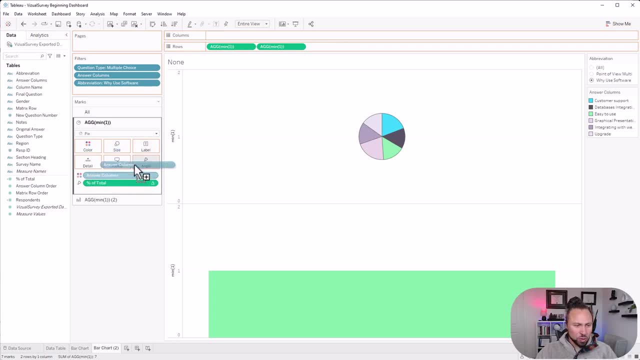 I'm going to add some labels, So I'm going to put: I'm going to make sure you hold control, because control duplicates the pillar, else You're going to mess up and move it. Hold control, Put that in the labels, All right. so we got pretty much the top done. 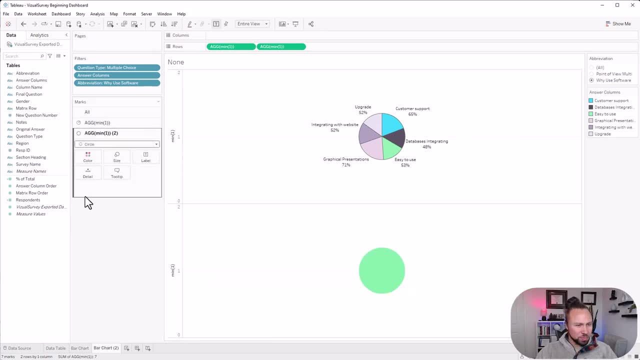 Now the bottom is: you Just do a circle, All right, we're just going to do a white and we're going to do a border And we're going to make it a little smaller, and we're going to have to play with this some. 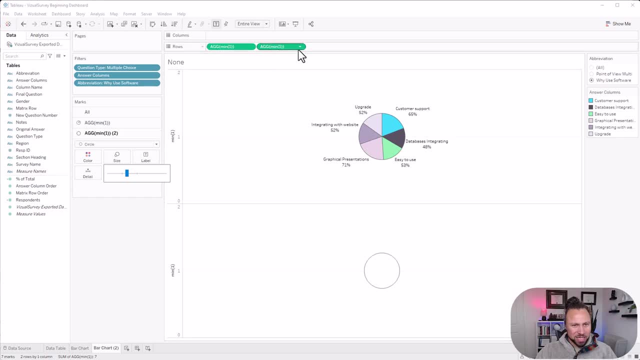 But what we're going to do is now just do, just do a dual axis and stack these on top of each other. So I'm going to go here, do dual axis and it just stacks it on top. So it looks like a pie chart, right? 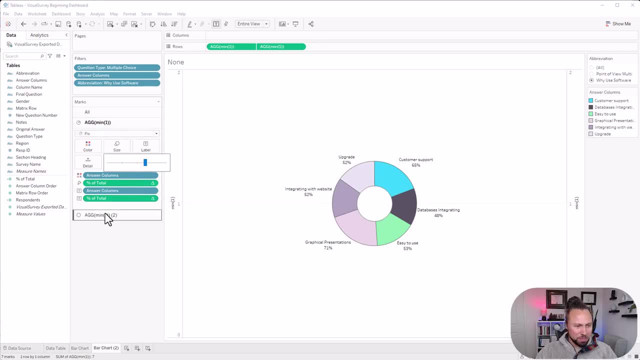 It is. We just got trick tableau into building one for it, So I'm going to play with the size until I get a good size I like. All right, that looks good. And now we got all these lines everywhere that you want to get rid of. 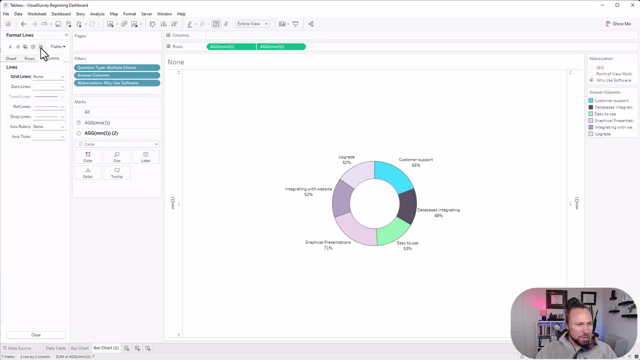 So just right-click and format up. here You have. you have your different lines. So you got column dividers You want to get rid of, probably, and then you got this line going across. I don't want. I'm going to get rid of my headers to on when I'm at it. 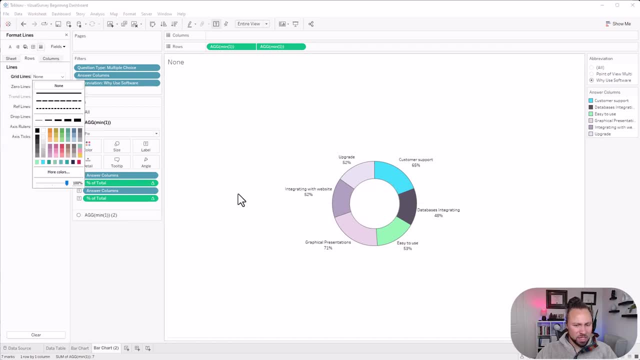 And that's these the grid line, I believe, Yeah, that's the grid line. So now we got a kind of nice, clean, clean Look, and then I mean that's pretty much it Like that's the donut chart. You can also add, for example, like your respondent counts, in your tooltips, if you like. 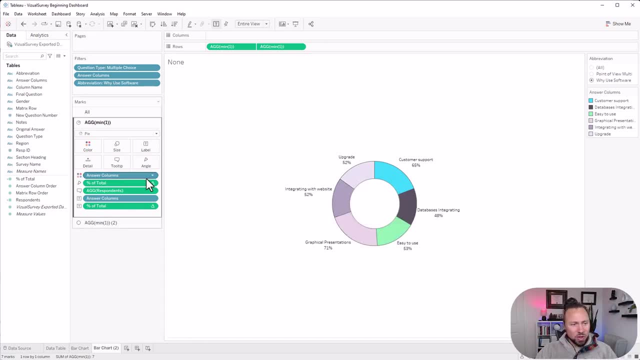 So I could put that on my tooltips. You want to see the respondent counts and then you can go in here and clean up your tooltips. So you don't need this. You just call this answers, if you like, So you can kind of clean it up. play with that. 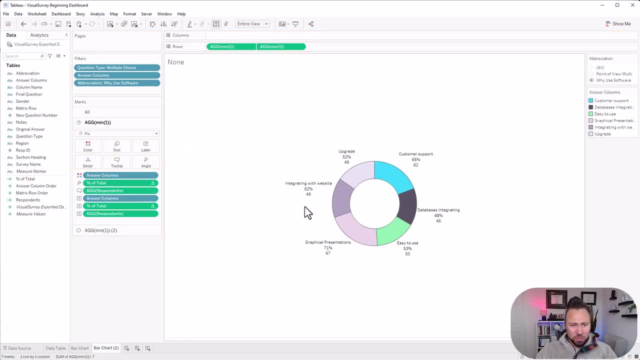 You could put your, your respondents, in your labels too, If you want to show that, and then you can go in here and play with this. Some sometimes I do this, and I'll maybe do hard code parentheses, something like that, or italicize it, So you can kind of see what's going on. 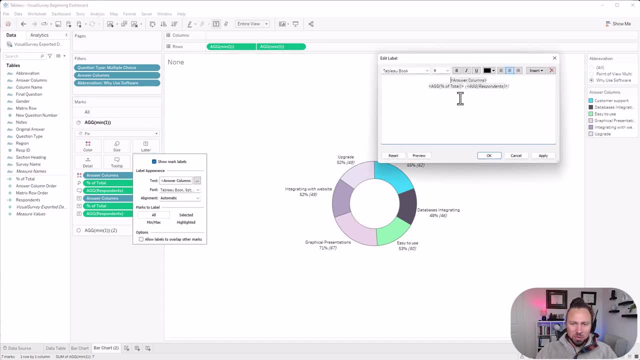 It's up to you, However. you want to really look at it or you can make you know this a little bigger. I mean, as you know probably, if you can deal with tableau, there's a million different features you can play with in tableau. 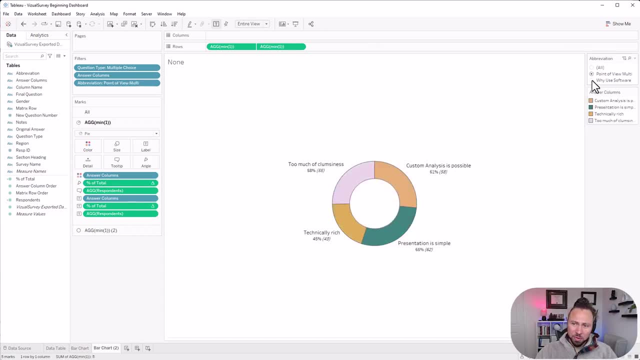 Okay, but that same thing and this works for all of them. Okay, you might have to play with the coloring some, because it's you assign colors in each, So you might have to go In here play with coloring, but but that's pretty much how you would do a doughnut chart. 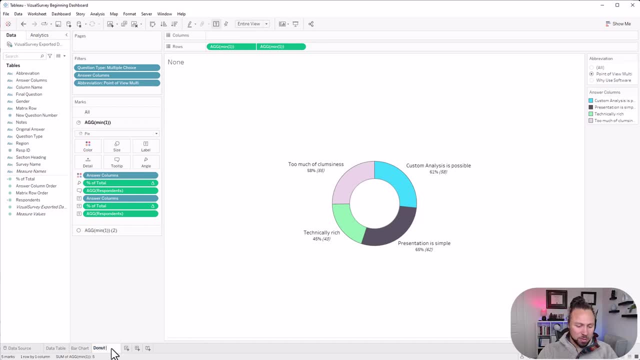 So you can either do this doughnut chart like this, You could do the regular bar chart, you could do text table, or we could do one more with that. I like doing whatever I like splitting data. Okay, because usually you want to like segment data. 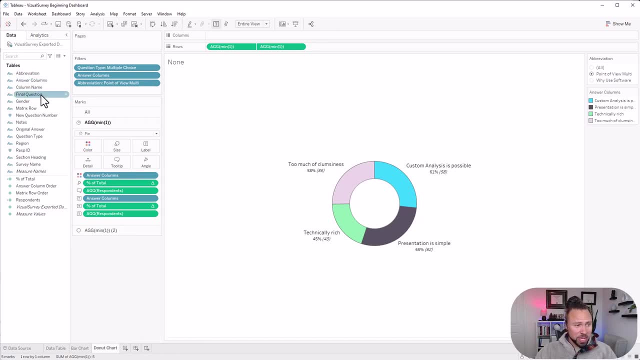 Sometime you want to see, all right Well, how it smells. a females look, which you can do like this. So if I bring gender out and put it in columns, I split it out right now. This is, this is. this is Knowles. 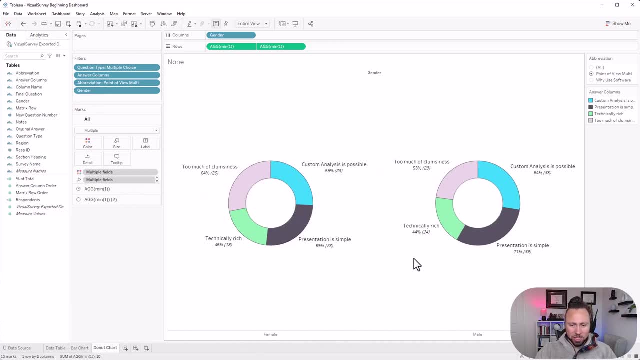 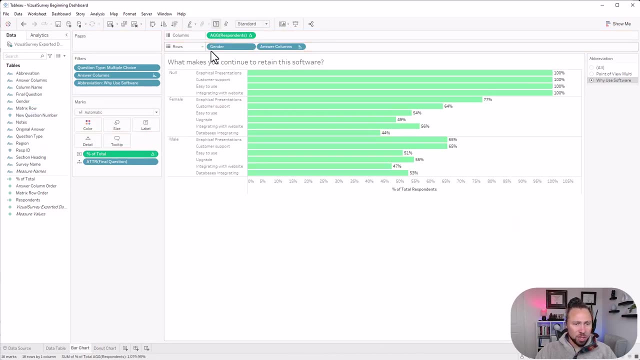 So somebody to answer it. We can get rid of this right, but now I have two pie charts, one for male, one for female. same thing for the, the bar chart. You can put this into rows or columns and segment it right, or you can put this into color and create like a stacked bar chart. 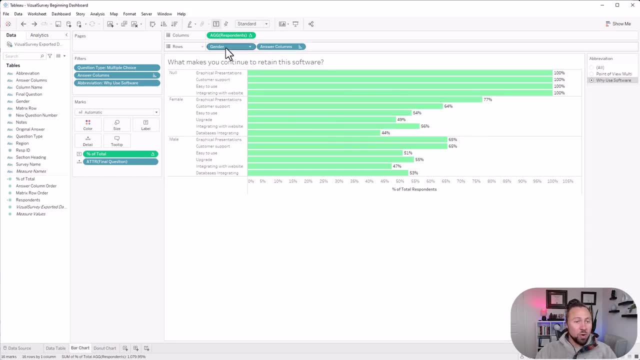 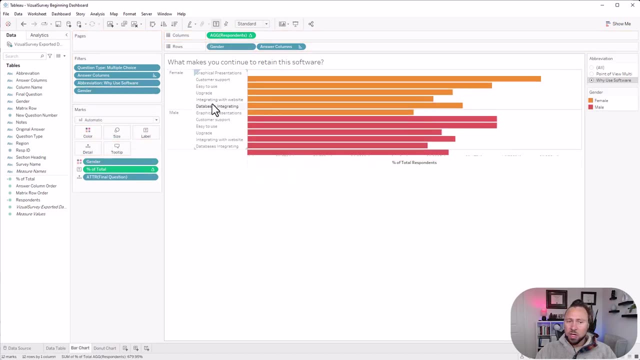 You have to play with that a little bit, but that's what we're going to do in the next one. or you could put leave it like this and hold control and put gender in a color and have two different ones, and then I exclude this right. 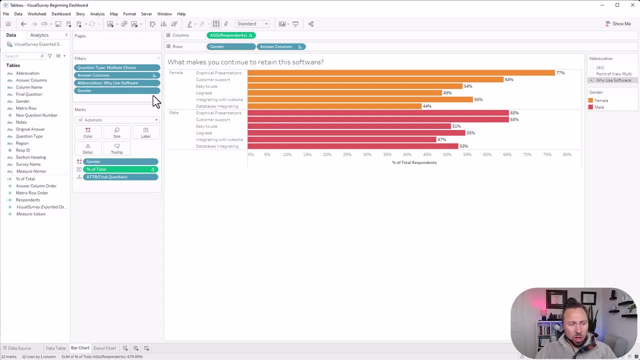 but the cool thing is, the data is in this perfect structure where you can do all this within a couple of clicks, and that's what makes visual survey So so powerful: because the data is already in a perfect structure. Now with with visual survey, 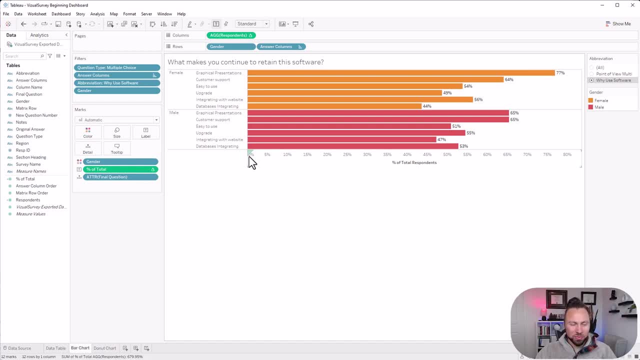 you already have all these dashboards built out for you, So you don't have to build all these from scratch. but you know, this is kind of cool way of getting some practice so that you can see kind of what's going on and how everything is working. 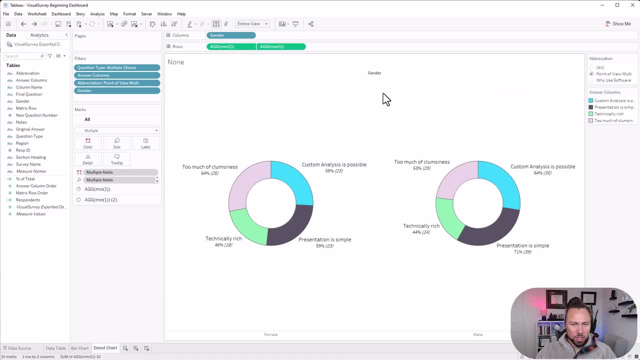 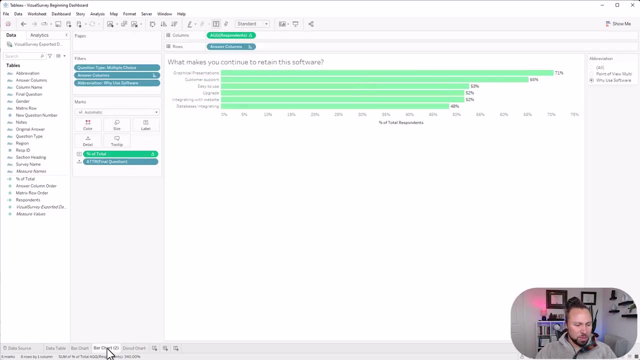 All right, so I'm going to undo some of this, so I get back to where I was and we're going to build one more. So let's go ahead and let's duplicate this bar chart, And we're going to use this to start off with now. 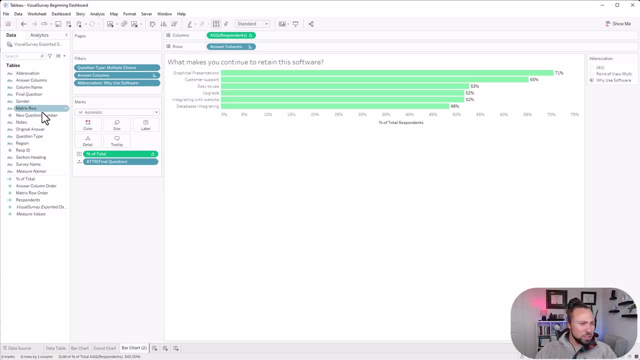 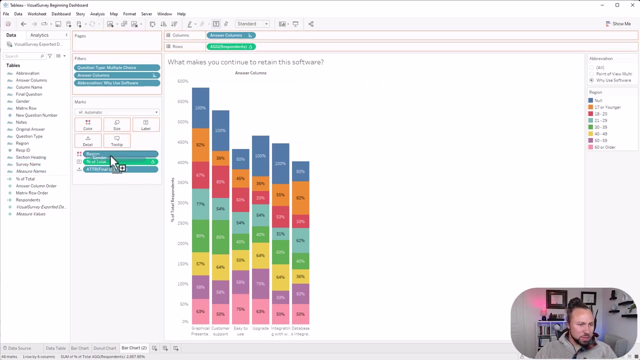 Let's say we want to put. let's put, let's put region into color- And I'm a flip, this actually- now let's put gender. that's too much going on. So we got gender. We have a knoll in there. We can get rid of that. 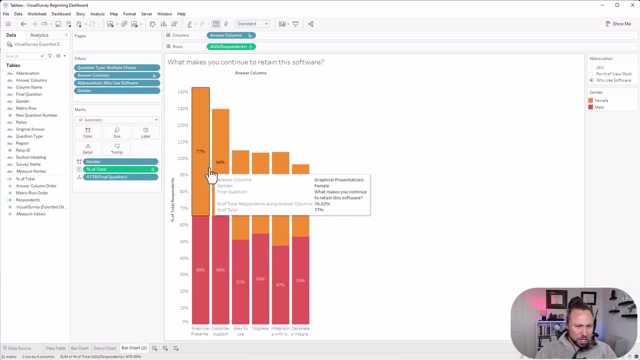 All right, so I can just click and exclude. Now we want to make sure that we're doing a percent of total going down Right, So let's just double check it. It should be it, but let's see. So it needs to be on answer columns. 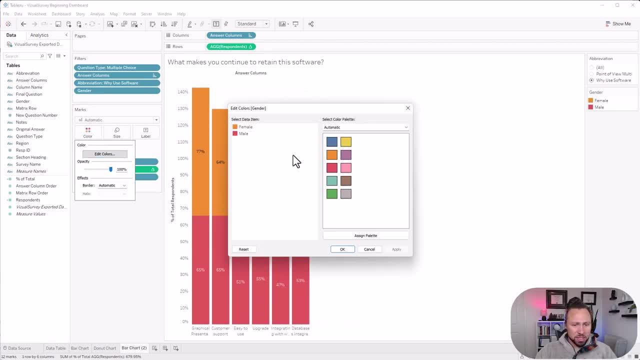 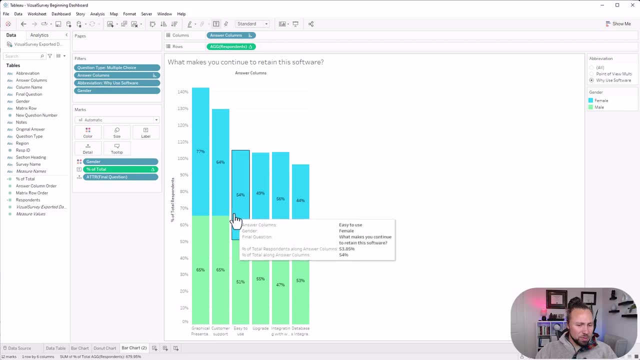 Okay, So, yeah, so we got our percent of total. could play with the coloring like this. I like using my colors, All right. we could play with the coloring like this, All right. and now we have this split up by a filter or something, right. 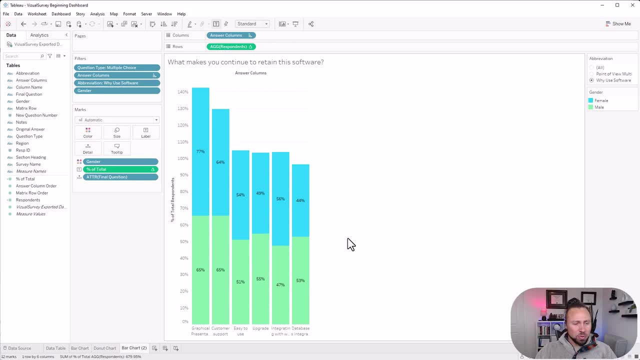 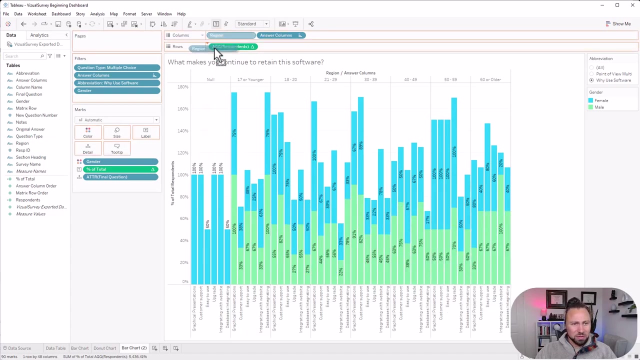 So we can see the difference between the two. We also can kind of play with it and add another, another one in. So let's grab or is it region? put that into columns and have this like segment it like this, And actually region is age. 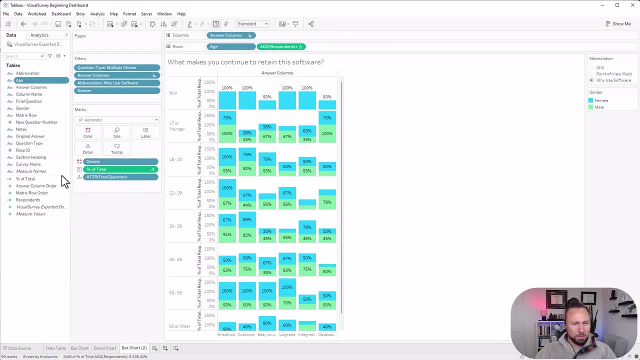 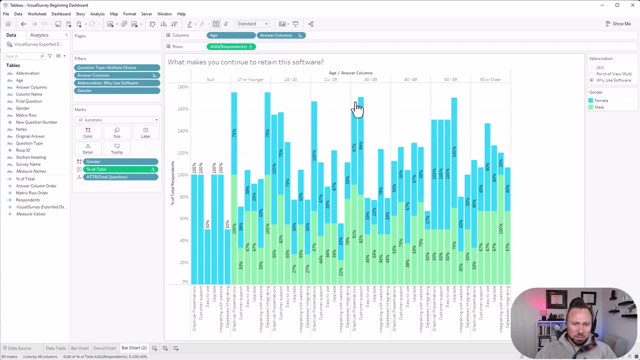 So let's go ahead and change that to age And we can have a segment out like that, Okay, and then you can kind of see the difference between all the ones. Now I'd probably change the coloring a little bit and or. 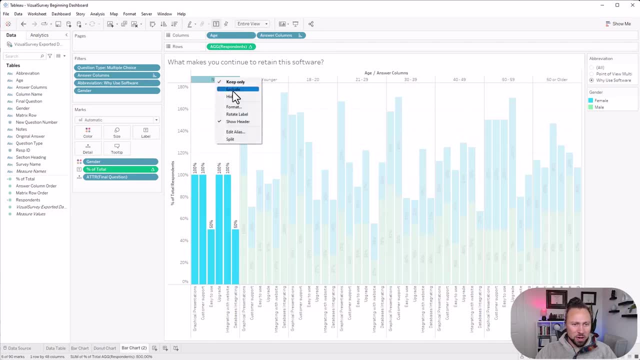 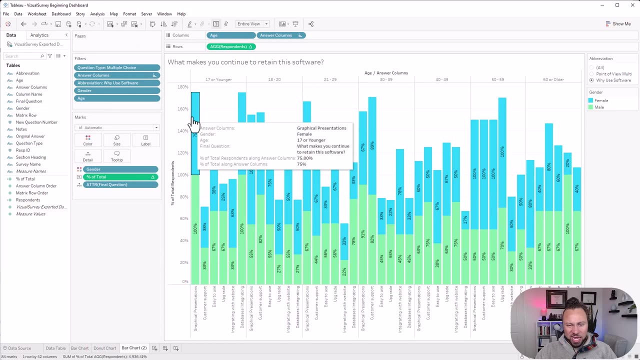 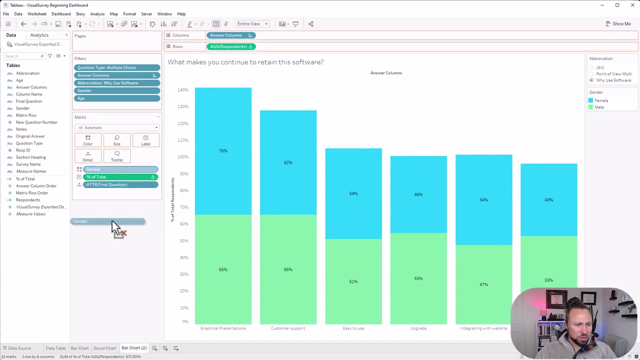 you know, maybe fit it, So it's a little better. Got to get rid of this knoll here. but you can now segment this data by by using another field to kind of cut it up. Another way we can do it is we can take out age. 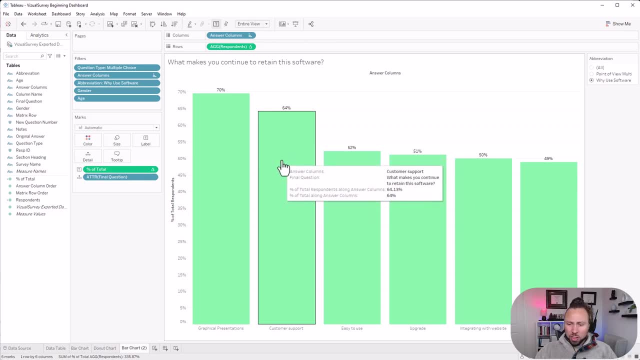 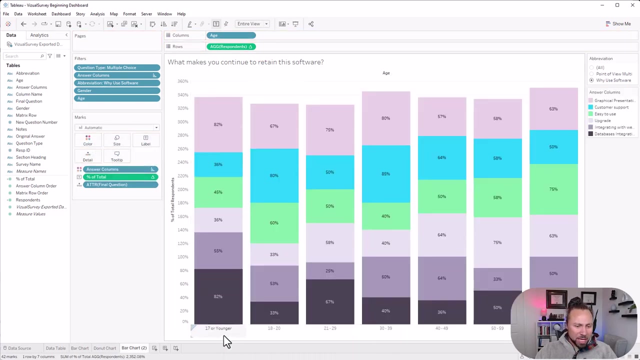 take out gender. All right, So we have our regular bar chart here. We can also put: let's grab Where's our age again. Okay, age here. Let's put answer columns into color instead. So we're kind of just swapping it right and now we can see all the different ages going across. our answer column is our ages or our answer column is our answers. 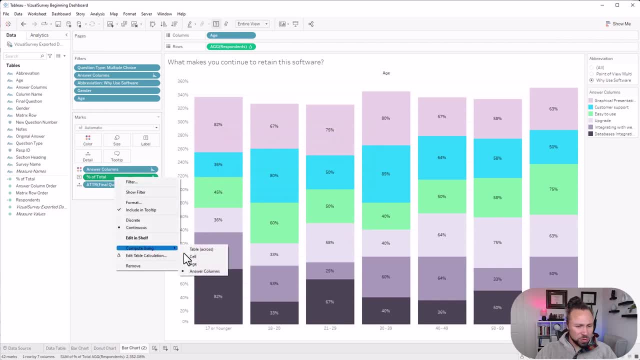 Okay, and we can make sure this, this percent of total Yep, It's on, Okay. So now we're looking for, you know, 17 or younger. This is how they answered: 18 to 20.. This is how I answered and we kind of see what the difference is between each, each age group. 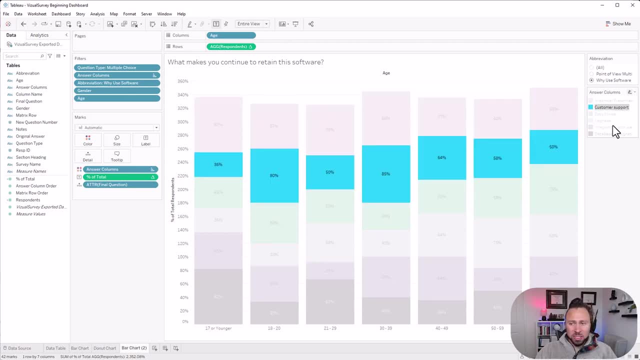 All right, So this is another cool way of looking at it. All right, So now, since we have the data structure, this way you can cut and slice the data in a lot of different ways. So this one- I'm just going to call this a stacked bar chart. 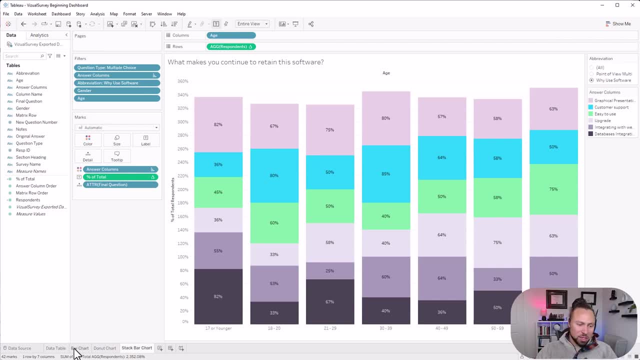 but this is used whenever you want to segment the data. Okay, essentially it's like the the regular bar chart, but you can segment the data by either putting your answer columns in color, or you can put either age or gender in a color, or a mix and match of being able to put like age here and then we can grab gender and put that in the columns. 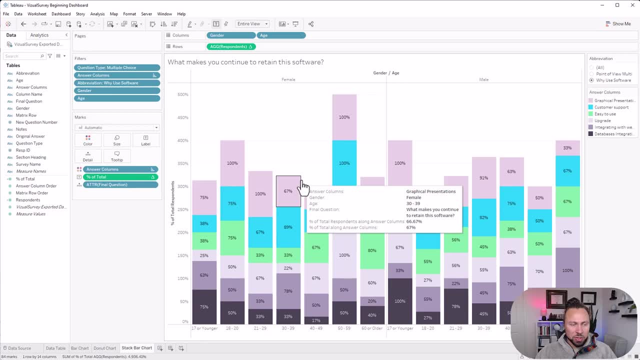 So you can play with this as much as you want and just clicking and dragging those pills into the different locations- Okay, but this is used whenever you want to compare a group of people. Alright, so we got the data table, We got the bar chart. 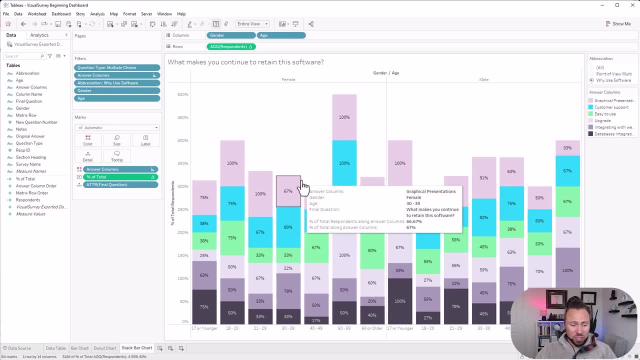 We have the donut chart and we have the stacked bar chart. All right, So these are the ones that I use the most when using multiple choice. If there is any other ones, I like to see it. I like to hear what it is. 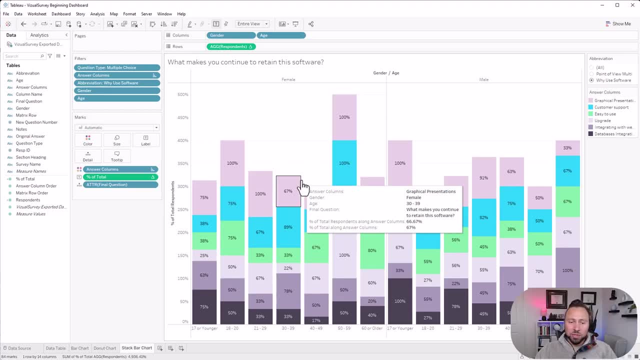 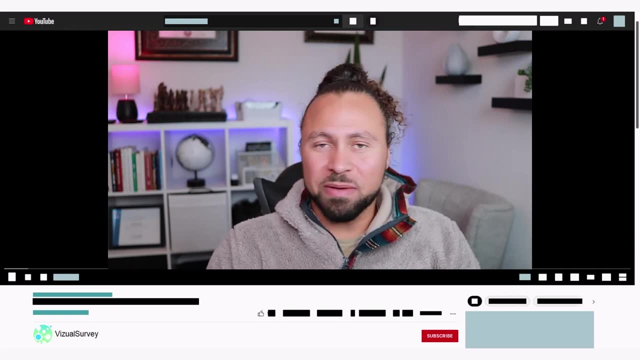 So please comment below what that is, But these are the ones I like doing the most. All right, Thanks for getting to the end of the video. As you saw, we have three different charts, including that text table, So four of ways we can analyze that data and visualize it, depending on how you want to look at it. 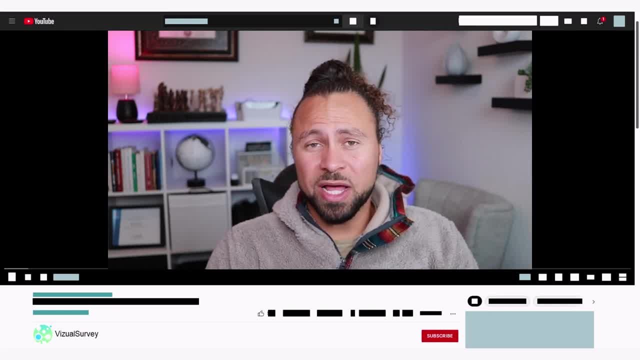 There's also, you know, a lot more. So if there's any charts that you like that I didn't cover in the multiple choice chart style kind of video, please comment down below of the chart style you like and then I will look at all the comments and probably make another video showing the different chart ways of doing that.